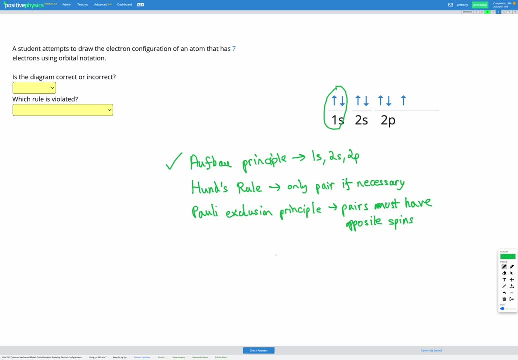 In the 1s energy level we just have one orbital, and so the electrons have to pair up as they go in there, So that part looks good. 2s again only has one orbital, so the electrons have to pair up as they go into there. That's our first four electrons. 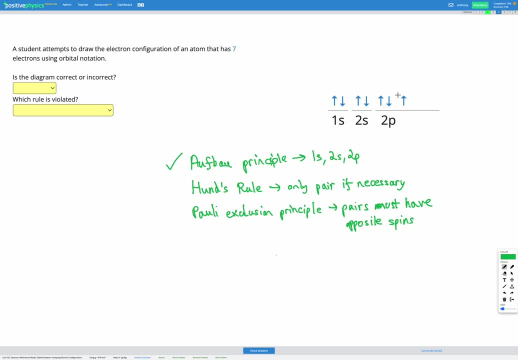 Next, in the 2p energy level there are three orbitals, because p sublevels can have three orbitals. Each orbital can fit up to two electrons. So we've got one, two, three orbitals available. So according to Hund's rule, the electrons should only pair up if they have to. 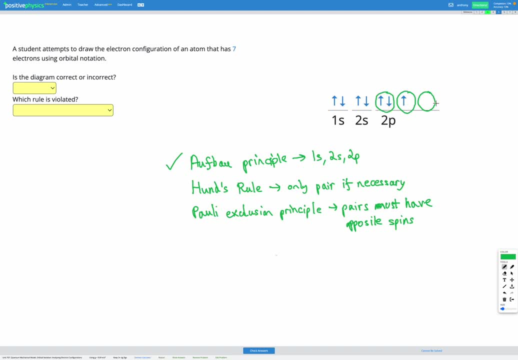 Here we've got two electrons paired and one on its own and one empty orbital. So this part isn't correct because this four is full. So we've got two electrons paired and one on its own and one empty orbital. The first pair of electrons didn't need to be a pair. This electron could have been. 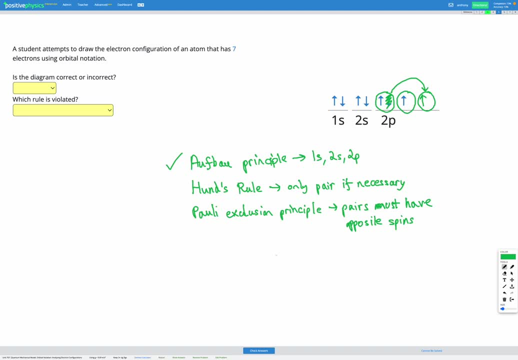 on its own in this orbital, and Hund's rule would then have been followed. But it wasn't, So Hund's rule has been violated here. Lastly, the Pauli exclusion principle says that pairs must have opposite spins. We've got three pairs in this diagram. All of them show arrows in opposite directions. 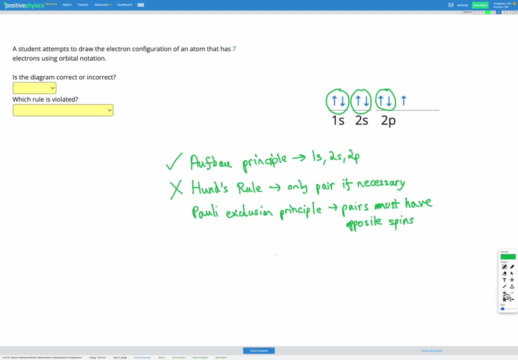 representing opposite spins. So we've got three pairs in this diagram. All of them show arrows in opposite directions representing opposite spins. We've got three pairs in this diagram. All of them show arrows in opposite directions representing opposite spins. So Pauli exclusion principle has been followed in this diagram. 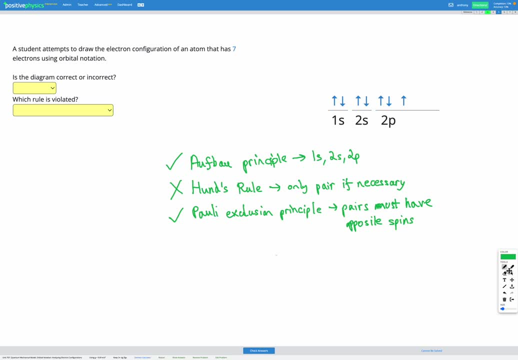 So overall it's not correct because Hund's rule has been violated In this question. we have an atom with four electrons, So let's go through and check if this student's diagram looks correct or not. Firstly, the Afbal principle: We have to fill the 1s subshell first. 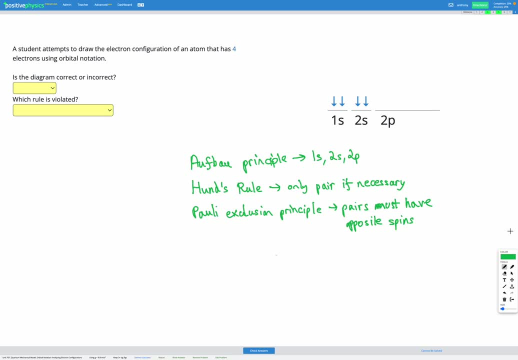 Then the 2s subshell and then the 2p subshell, etc. Here we can see we've got two in the 1s subshell, so that's full, Two in the 2s subshell, so that's full, and that's all our electrons. 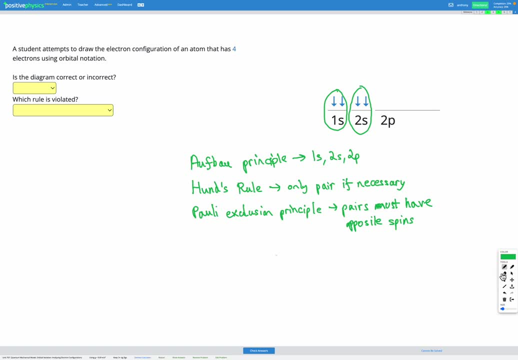 So that looks correct. they filled in the right order. So Afbal principle is being followed. Hund's rule is that electrons should only pair if necessary. So on our first sublevel we have one orbital that can fit two electrons, So those two have to pair.